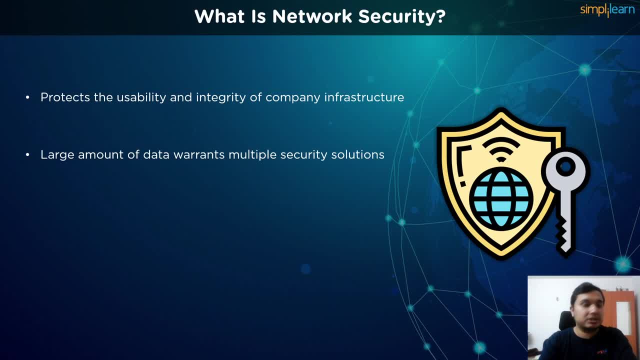 It has the network the user chooses. Recently, network security has become the central topic of cybersecurity, with many organizations involving applications from people with skills in this area. It is crucial for both personal and professional networks. Most houses with high speed internet have one or more wireless routers, which can be vulnerable to attacks. 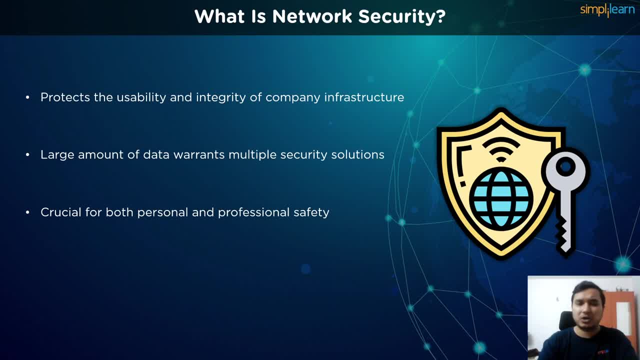 if they are not adequately secured. Data loss, theft and sabotage risk may be decreased with the usage of a strong network security system. The workstations are protected from hazardous firewall thanks to network security. Additionally, it guarantees the security of the data which is being shared over a network By dividing information into various sections. 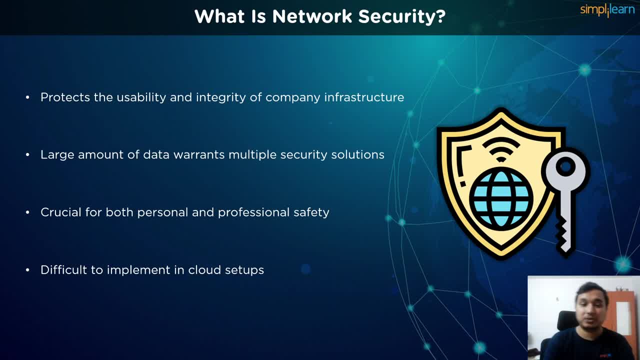 encrypting these portions and transferring them over separate pathways. network security infrastructure offers multiple levels of protection. Network security can be used to thwart man-in-the-middle attacks, preventing situations like eavesdropping, among other harmful attacks. It is becoming increasingly difficult in today's hyper-connected 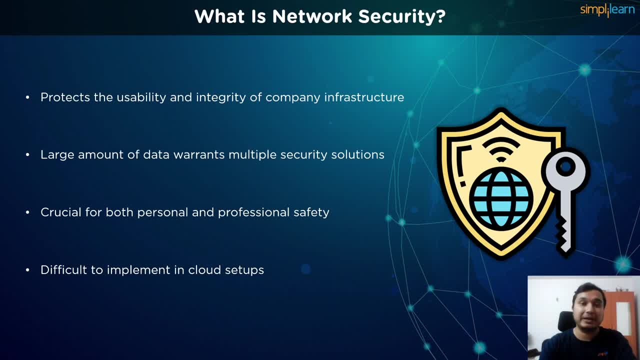 environment as more corporate applications migrate to both public and private networks. Additionally, modern applications are also frequently virtualized and dispersed across several locations, some outside the physical control of the IT team. Network traffic and infrastructure must be protected in these cases, since assaults on businesses are increasingly. 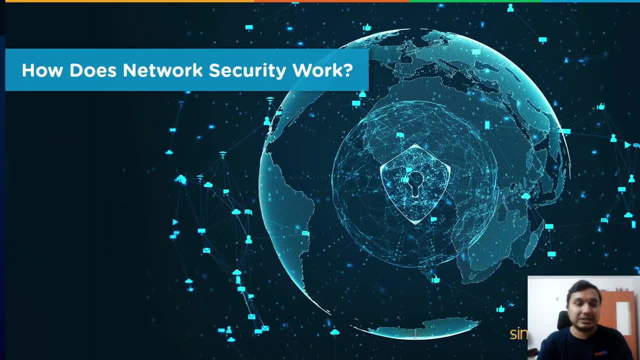 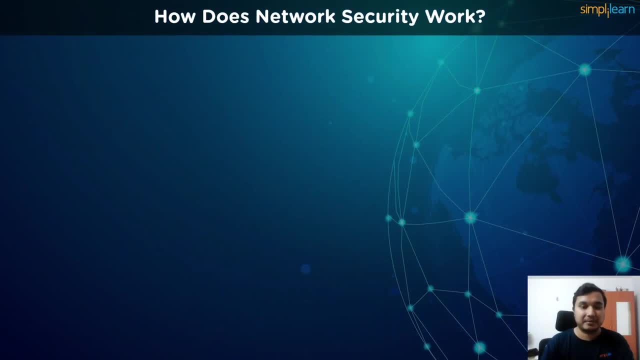 common. We have now understood the basics of network security, but we need to understand how network security works. in the next section, in slightly more detail, Network security revolves around two processes: authentication and authorization. The first process, which is authentication, is similar to access paths which ensure that only those 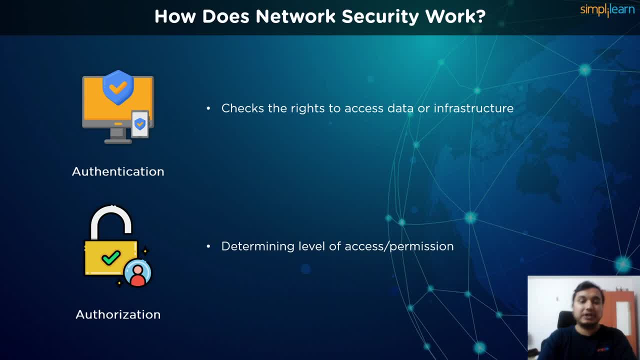 who have the right to enter a building. In other words, authentication checks and verifies that it is indeed the user belonging to the network. Next comes authorization. This process decides the level of access provided to the recently authenticated user. For example, the network admin needs access to the entire network. 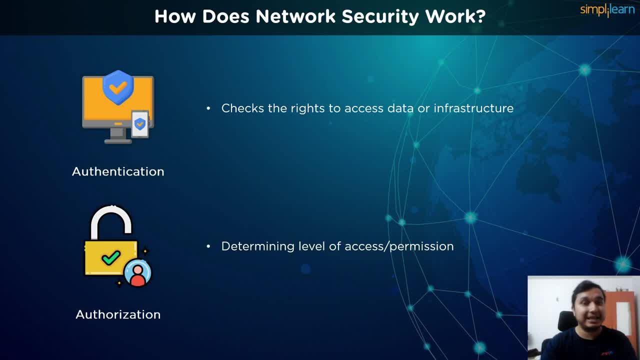 whereas those working within it probably need access to only certain areas within the network. Based on the network user's role, the process of determining the level of access or permission level is known as authorization. Next comes authorization. This process decides the level of access provided to the recently. 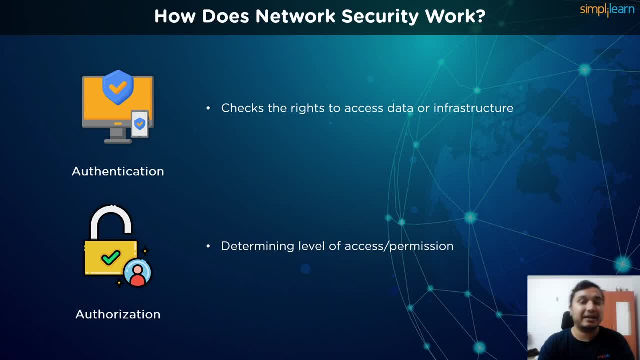 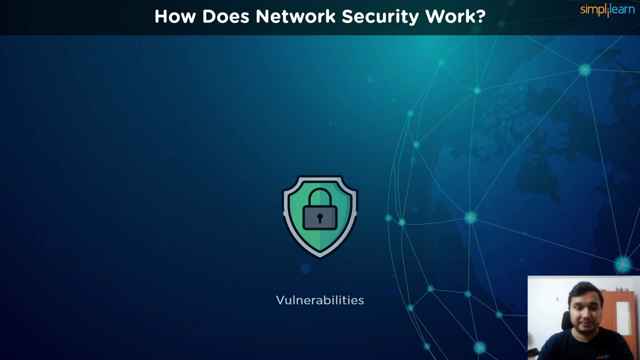 authenticated user. Today's network architecture is complex and faces a threat environment that is always changing and attackers that are always trying to find and exploit vulnerabilities. These vulnerabilities can exist in many areas, including devices, data, applications, users and locations. For this reason, many network security management tools and applications are in use today that 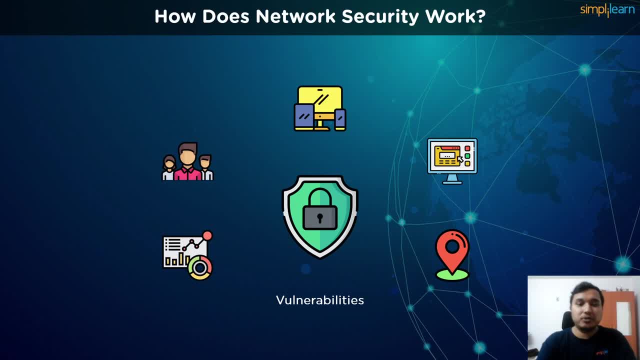 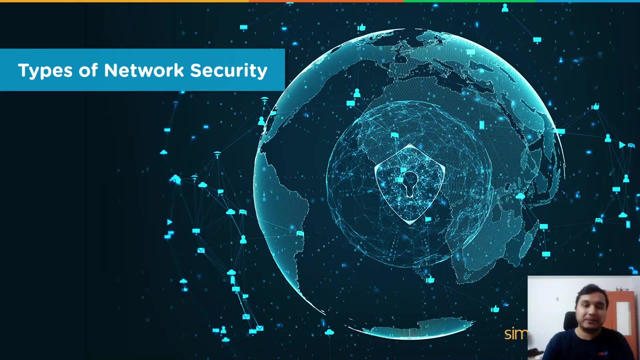 address individual threats. When just a few minutes of downtime can cause widespread disruption and massive damage to an organization's bottom line and reputation, it is essential that these protection measures are in place beforehand. Now that we know a little about network security and its workings, let's cover the different. 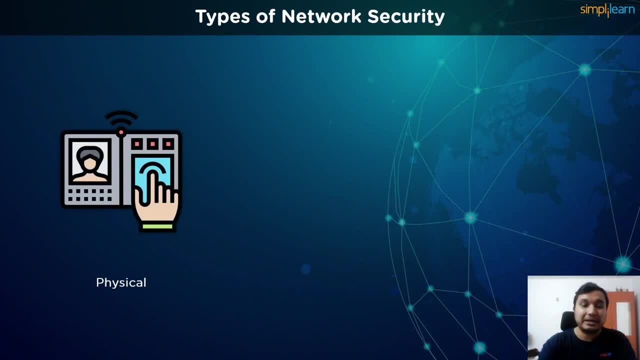 types of network security. The fundamental tenet of network security is the layering of protection for massive networks and stored data that ensure the acceptance of rules and regulations As a whole. there are three types, The first of which is physical security, The next being security and security. 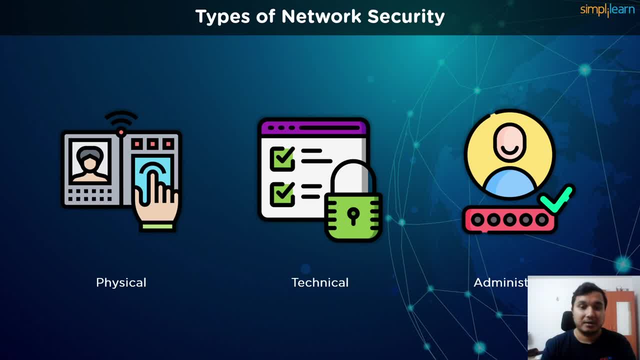 being technical and the third being administrative. Let's look into physical security first. This is the most basic level. that includes protecting data and network to unauthorized personnel from acquiring control over the confidentiality of the network. This includes external peripherals and routers that might be used for cable connections. 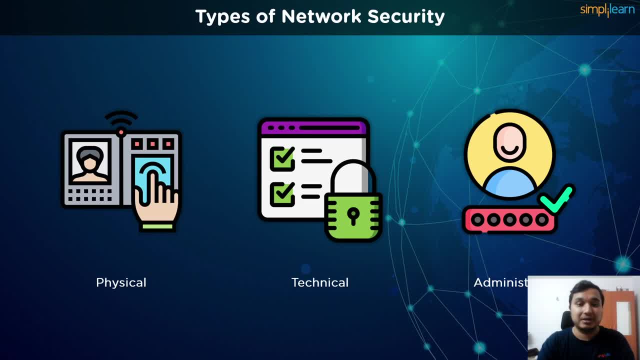 The same can be achieved by using devices like biometric systems. Physical security is critical, especially for small businesses that do not have many resources to devote to security. When it comes to technical network security, it focuses mostly on safeguarding data either kept in the network or engaged in network transitions. This kind fulfills two functions. 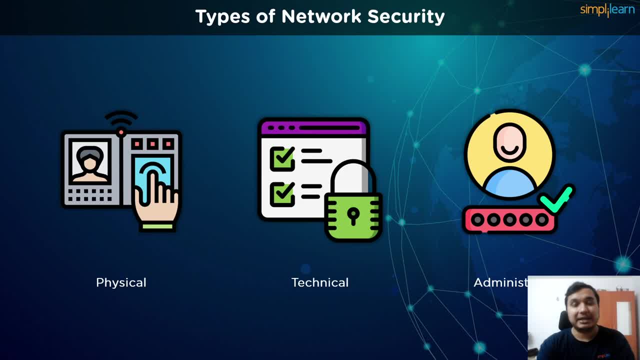 One is defense against unauthorized users. The other is a defense against malevolent actions. The last category is administrative. This level of network security protects user behavior, like how the permission has been granted and how the authorizes the user to use the data. 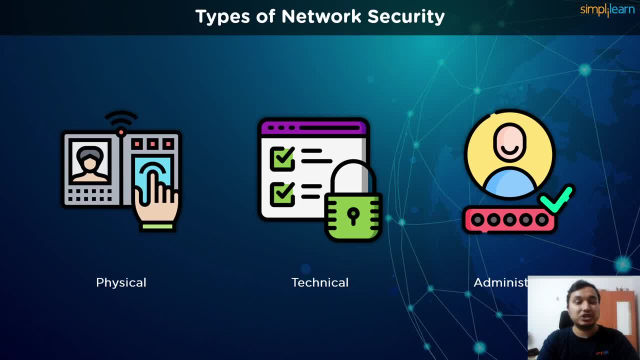 As an example, It is necessary to talk about the trust and privacy of the users and how the authorization process takes place. This also ensures the level of sophistication the network might need to protect it through all attacks. This level also suggests necessary amendments that have to be done to the infrastructure. 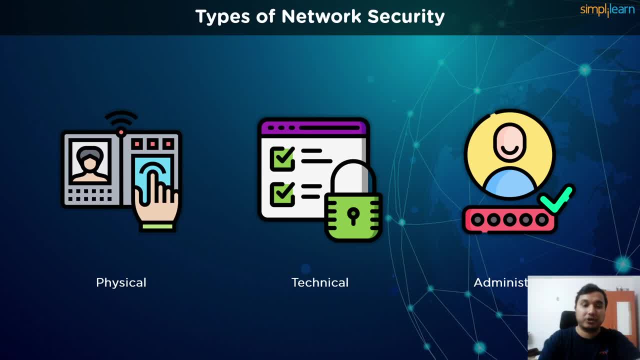 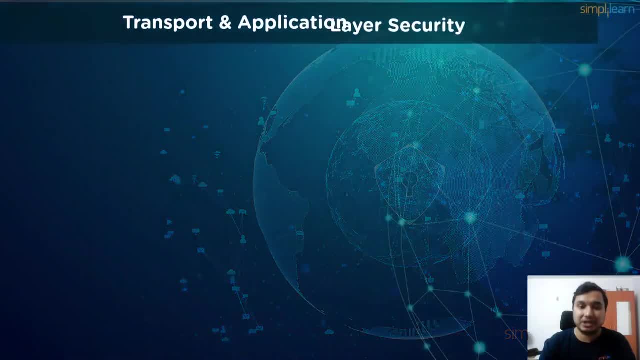 I think here are the basics that we need to cover on network security. In our next topic we are going to go through two mediums of network security, which are the transport layer and the application layer. The transport layer is a way to secure information as it is carried over the Internet, For example. 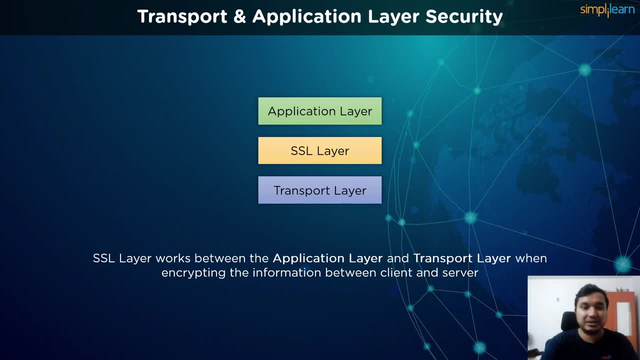 with users browsing websites, emails, instant messaging, etc. TLS aims to provide a private and secure connection between a web browser and a website server. It does this with a cryptographic handshake between two systems using public-key cryptography. The two parties to the connection exchange a secret token. 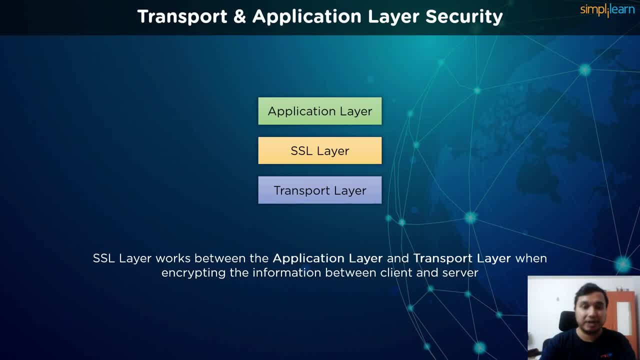 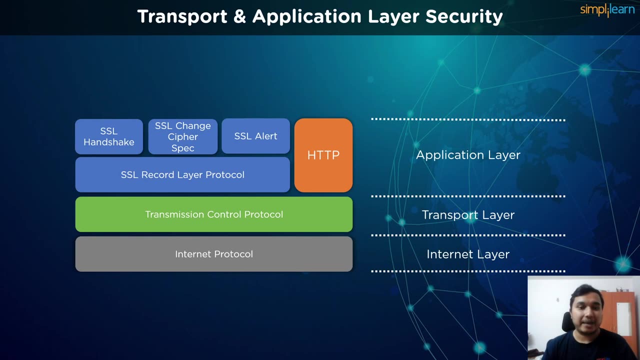 and once each machine validates this token, it is used for all communications. The connection employs lighter symmetric cryptography to save bandwidth and processing power. Since the application layer is the closest layer to the end user, it provides hackers with the largest threat surface. Poor app layer security can lead to performance and stability issues. 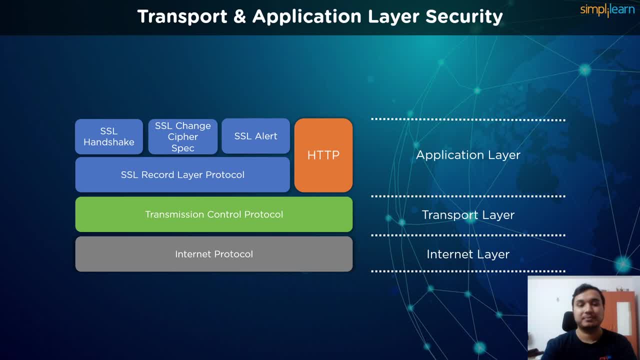 data theft and, in some cases, the network being taken down. Examples of application layer attacks include distributed denial-of-service attacks or DDoS attacks, HTTP floods, SQL injections, cross-site scripting, etc. Most organizations have an arsenal of application layer security protections. 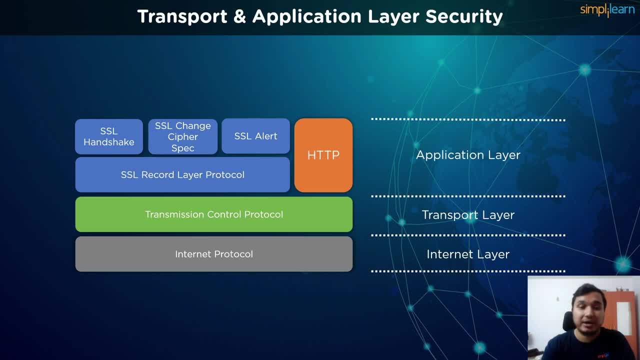 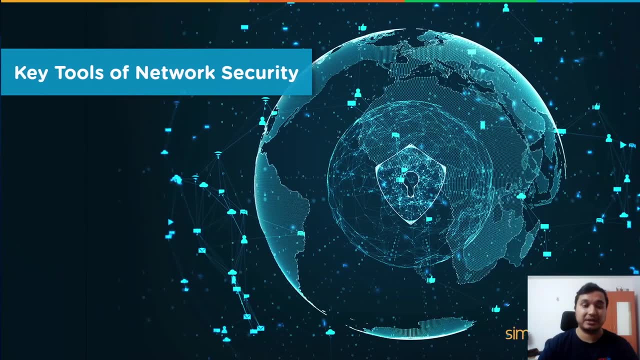 to combat these and more, such as web application firewalls, secure web gateway services, etc. Now that we have the theory behind network security has been covered in detail, let us go through some of the tools that can be used to enforce these network security policies. 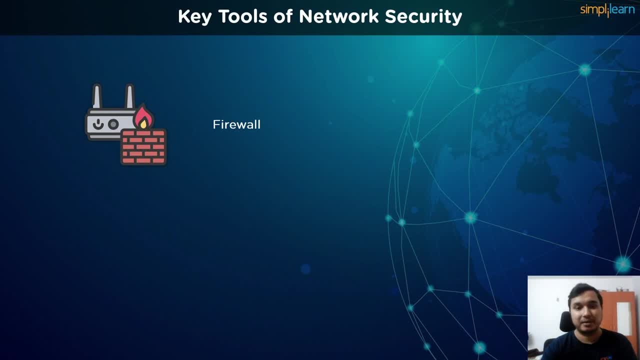 The first tool to be covered in this section is a firewall. A firewall is a type of network security device that keeps track of incoming and outgoing network traffic and it decides which traffic to allow or deny, in accordance to a set of security rules. 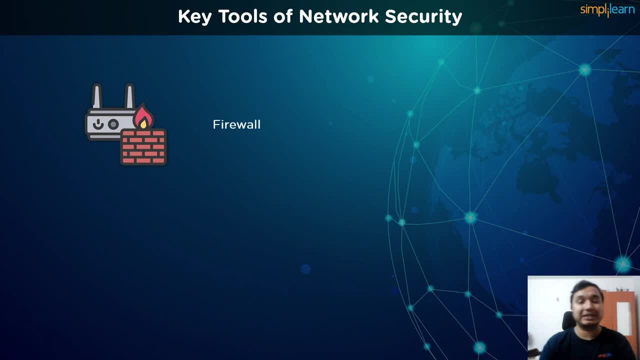 For more than 25 years, firewalls have served as network security's first line of defense. They provide a barrier between trustworthy internal, protected and regulated networks from shady external networks like the internet at some point. The next tool which can be used to bolster network security is a virtual private network. 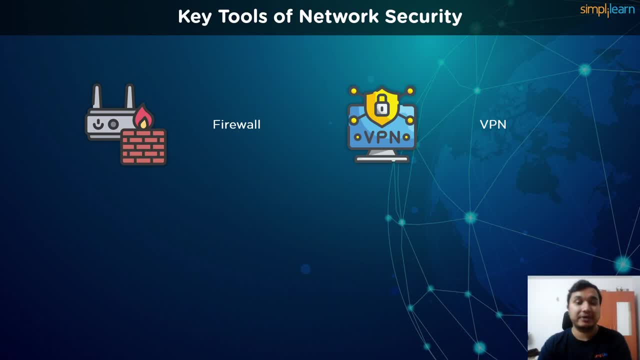 or VPN for short. It's an encrypted connection between a device and a network via the internet. The encrypted connection aids the secure transmission of sensitive data. It makes it impossible for unauthorized parties to eavesdrop on the traffic and enables remote work for the user. 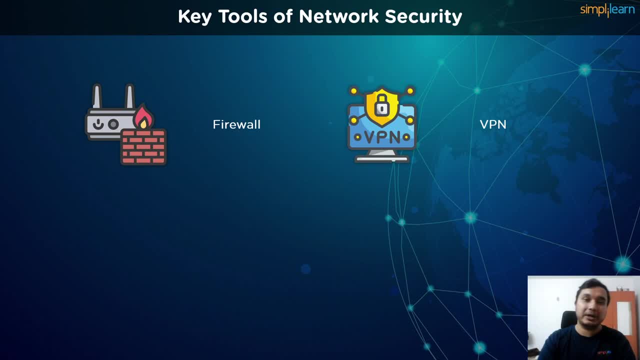 The usage of VPN technology is common in both corporate and personal networks. Next, we cover the importance of intrusion prevention systems in network security, or IPS frameworks. An intrusion prevention system is a network security tool that continually scans a network for harmful activity and responds to it when it does occur. 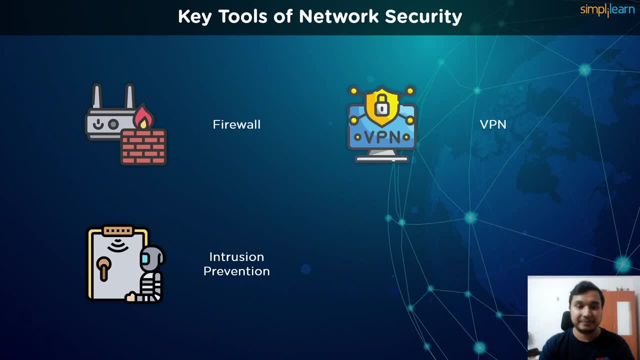 By reporting, blocking or discarding it. It can be either hardware or software. It's more sophisticated than an intrusion detection system or an IDS framework which can just warn an administrator and merely identify harmful activities, while in the case of an IPS, it actually takes against that activity. 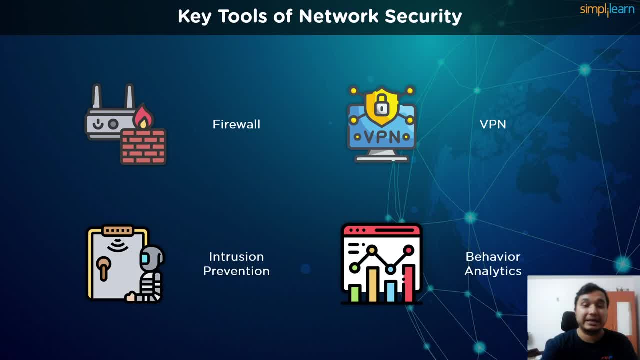 The next tool in this section, and the final one, are going to be behavioral analytics. Behavioral analytics focus more on the statistics that are being carried over and stored through months and years of usage. Once some kind of similar pattern is noted, where the IT administrator can detect some. 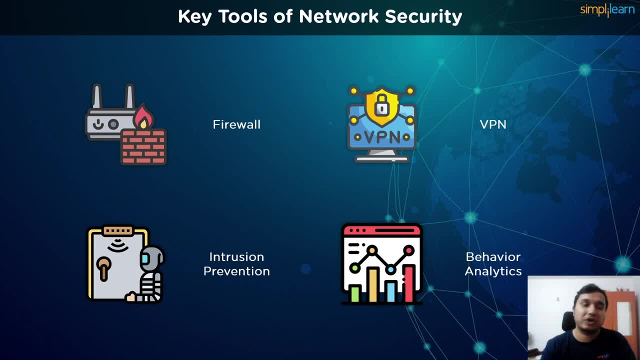 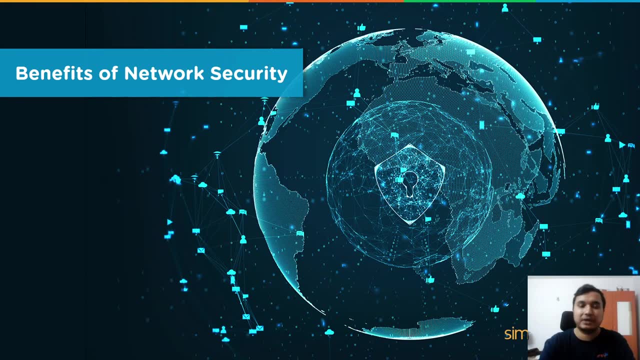 kind of attack. the similar attacks can be stopped and the security can be further enhanced. Another way of covering all that we need to know about network security, the necessary tools, its different types, etc. Let's go through the benefits of network security as a whole. 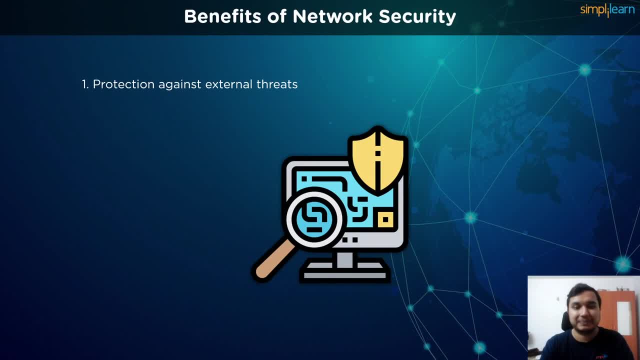 The first, which is protection against external threats. The objective for cyber assaults can be as varied as the defenders themselves, Although they're typically initiated for financial gain. whether they are industrial spies, hacktivists or cyber criminals, these bad actors all have one thing in common: 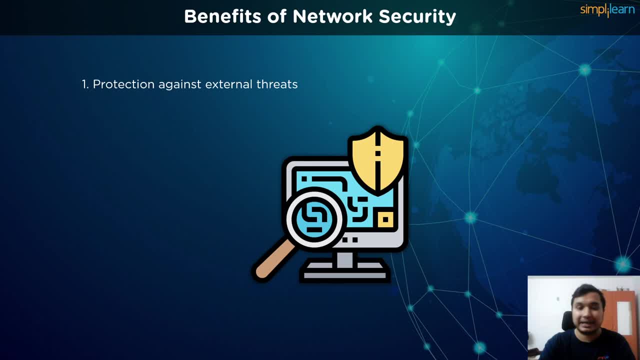 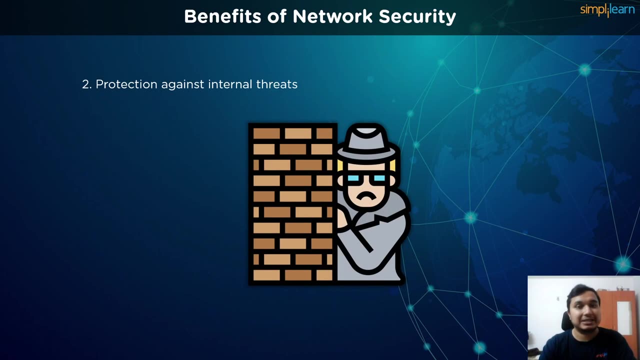 which is how quick, clever and covert the attacks are getting. A strong cybersecurity posture that considers routine software updates may assist firms in identifying and responding to the abuse, techniques, tools and the common entry points. The next benefit is protection against internal threats. 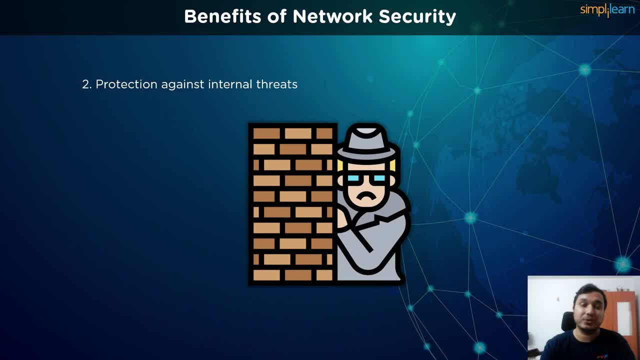 The human aspect continues to be the cybersecurity system's role, system's weakest link. Insider risk can originate from current or former workers, third-party vendors or even trusted partners, and they can be unintentional, careless or downright evil. Aside from that, the rapid expansion of remote work and the personal devices used for business, 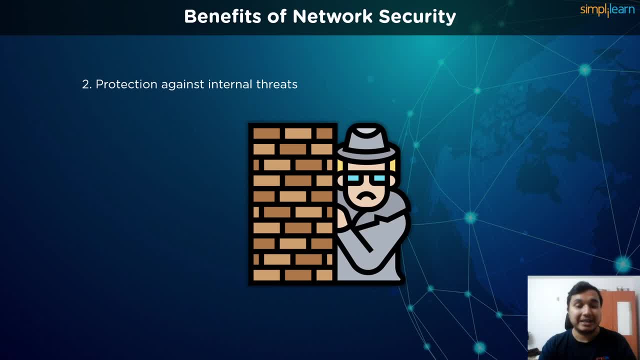 purposes, while even IoT devices in remote locations can make it easier for these kind of threats to go undetected until it's too late. However, by proactively monitoring networks and managing access, these dangers may be identified and dealt with before they become expensive. 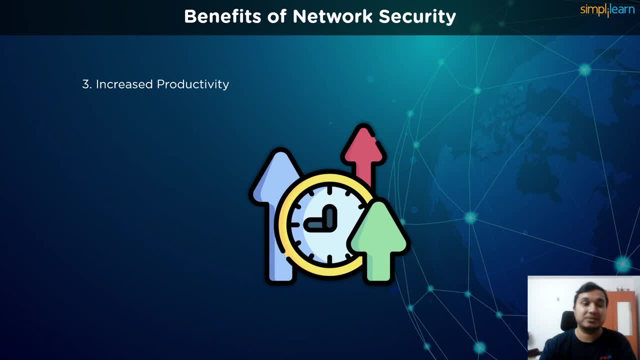 disasters. The third benefit is increased productivity. It is nearly impossible for employees to function when networks and personal devices are slowed to a crawl by viruses and other cyber attacks during the operation of website and for the company to run. You may significantly minimize violations and the amount of downtime required to fix the breach by implementing various 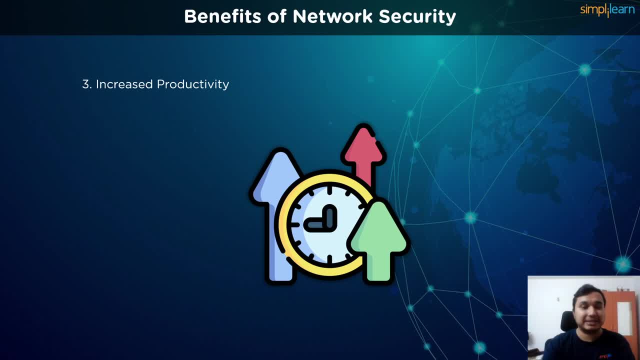 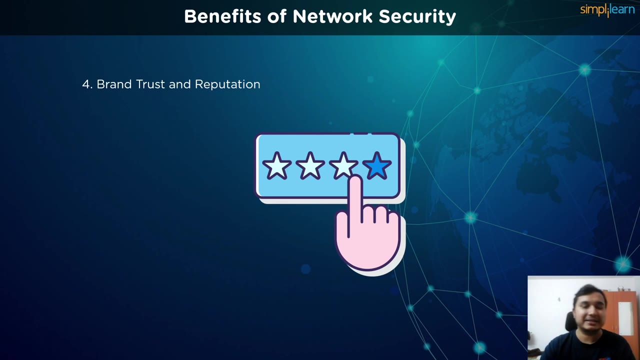 cybersecurity measures such as enhanced firewalls, virus scanning and automatic backups. Employee identification of possible email phishing schemes, suspicious links and other malicious criminal activities can also be aided by education and training. Another benefit is brand trust and reputation. Customer retention is one of the most 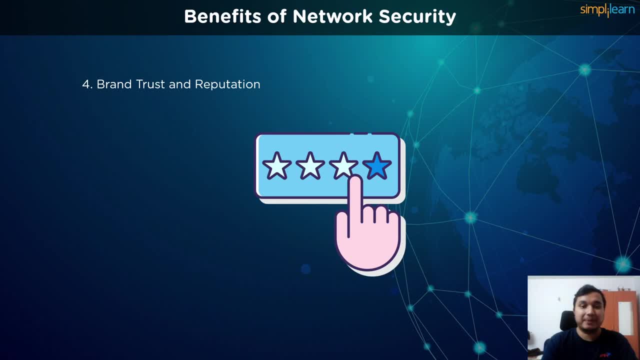 crucial elements in business development. Customers today place a premium on maintaining brand loyalty through a strong cybersecurity stance, because this is the fastest way to get other businesses back on track. This is a key takeaway from today's talk back: get referrals and sell more tickets overall. 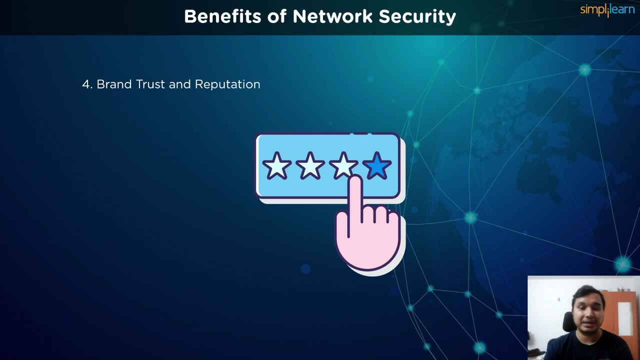 Additionally, it helps manufacturers get on the vendor list with bigger companies as a part of the supply chain, which is only as strong as its weakest link. This opens possibilities for potential future endeavors and development. That's all really for all, for the theoretical part. 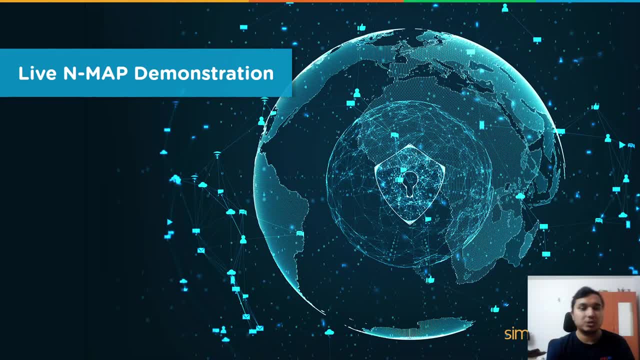 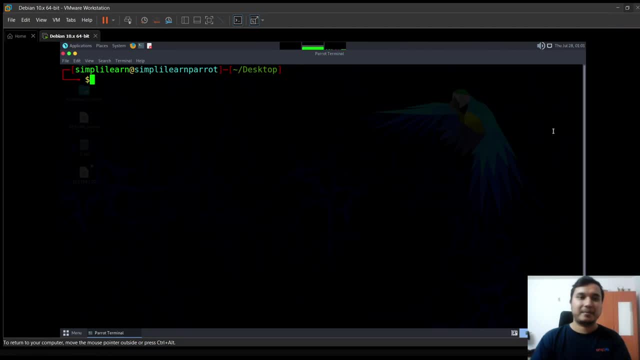 of network security. After covering so many topics, let's go through a small demonstration to drive home this topic's importance. So one of the first things we're going to cover is the installation of NMAP. What we're using right now is actually 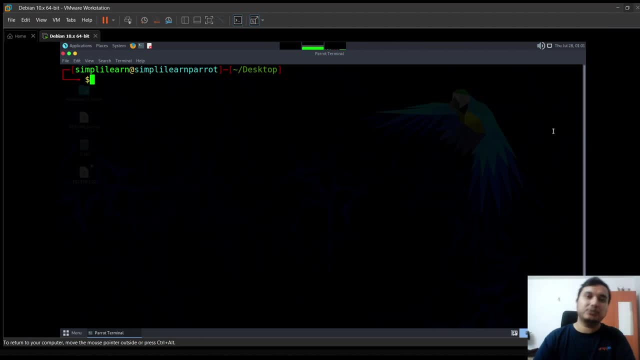 VMware, where we are running an instance of a Linux distribution known as Parallel Security Operating System. The Parallel Security OS is a Debian-based Linux distribution that is catered more towards ethical hackers and penetration testers. How it is catered more is it comes pre-installed with a lot of tools. 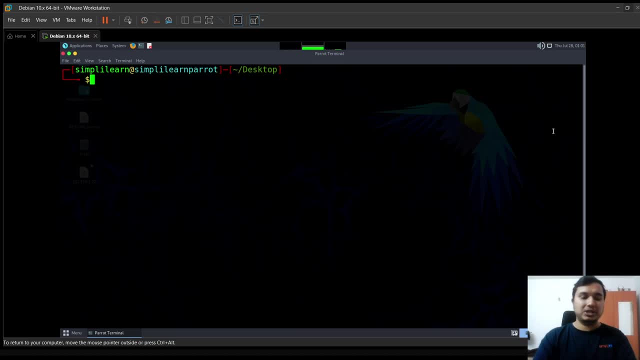 that ethical hackers need, including NMAP. So let's say you're using another Debian-based Linux distribution. If you want to install NMAP, you can go with the command of sudo apt, which is the package manager, Install NMAP And just press Enter. 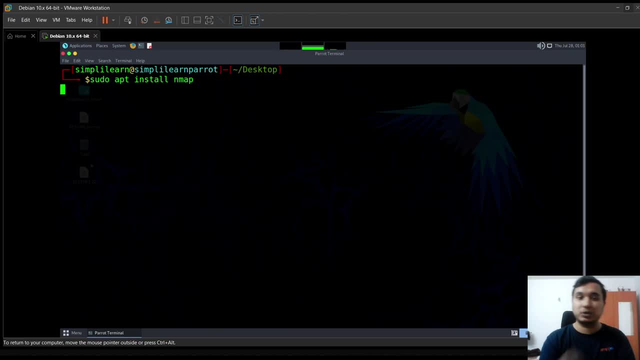 At this point it's going to ask you for your administrator password because of the sudo command which you have used. Now this apt will change depending on the distribution. Let's say, using a distribution that is based on Arch Linux, That will be different. 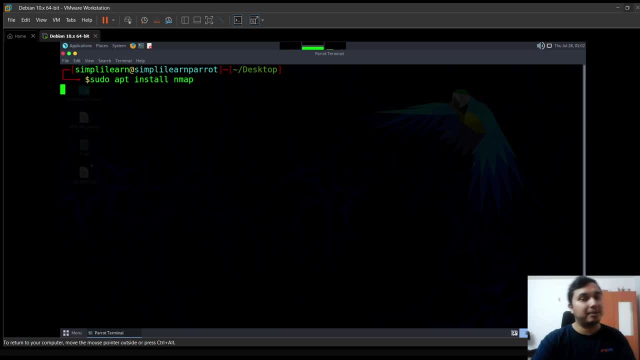 If there is some other distribution which is built from scratch, the commands will differ. But more or less a lot of the distributions, the mainstream distributions that people use, like Ubuntu, Zorin OS, MaxMint- they are Debian-based, So you're just going to be using sudo, apt install NMAP. 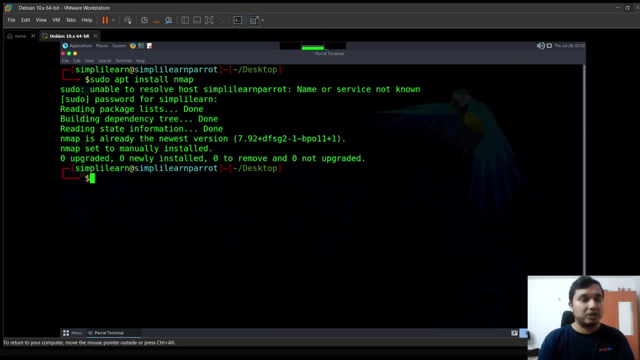 If you give your administrator password here, it's going to see that NMAP is manually installed and it is already the newest version At this point. if you do not have NMAP in your distribution, it's going to install the necessary package files. 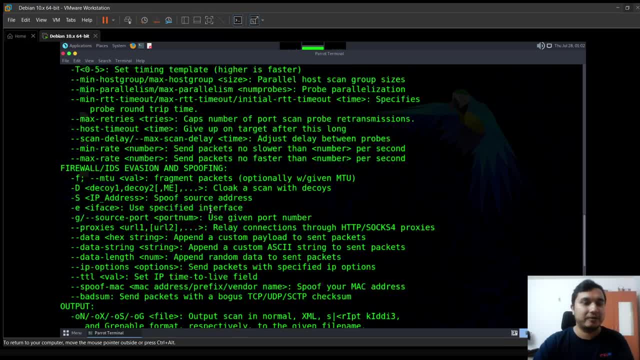 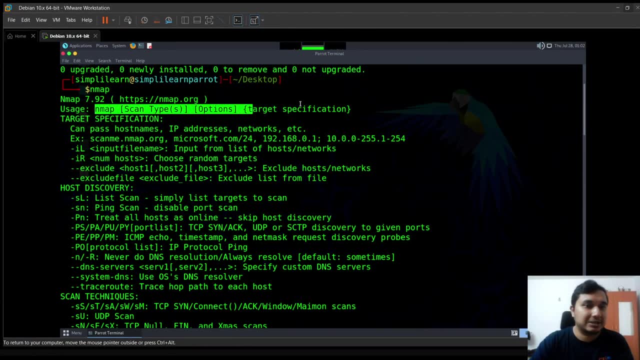 If I just use the NMAP command you can see some helplines where it's basically says what kind of flags you can use, what are some of the most common commands, the version, et cetera. It gives a small sample for the usage of NMAP. 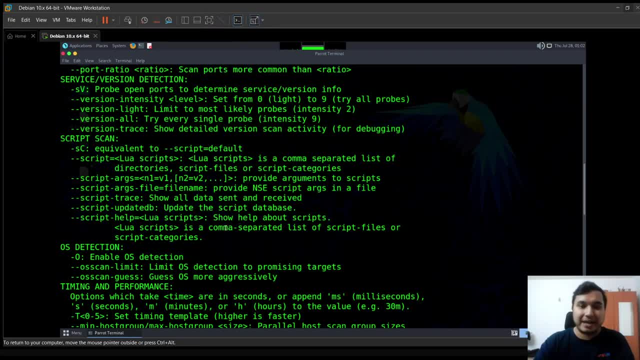 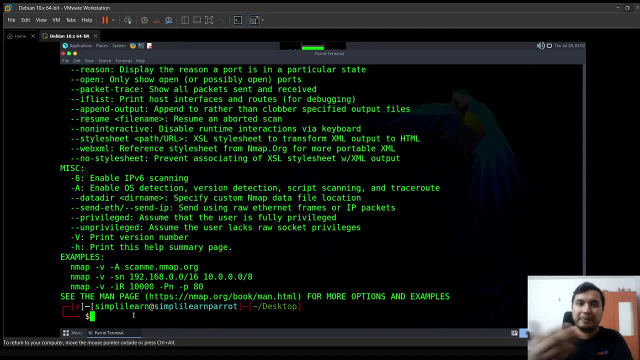 Now the first. one of the most basic functions of NMAP is to identify active hosts on your network. NMAP does this by using a ping scan, or sometimes it's called a ping sweep. This identifies all of the IP addresses that are currently online without sending. 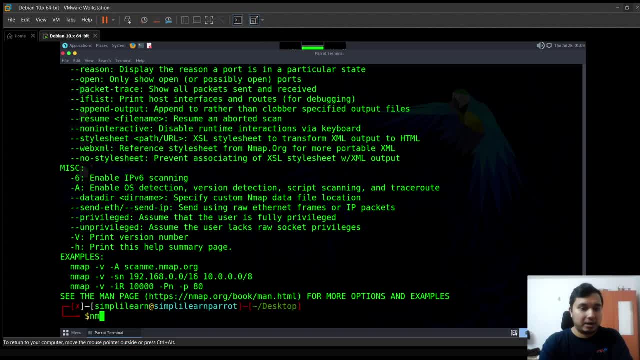 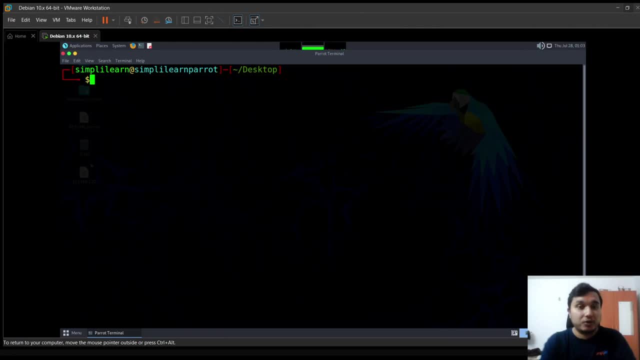 any packets to these hosts. To run the command, you need to use the command. we're just going to go with it. Let me just clear the screen for now. Another thing you have to do before running NMAP, just for our ease of use, is we're going. 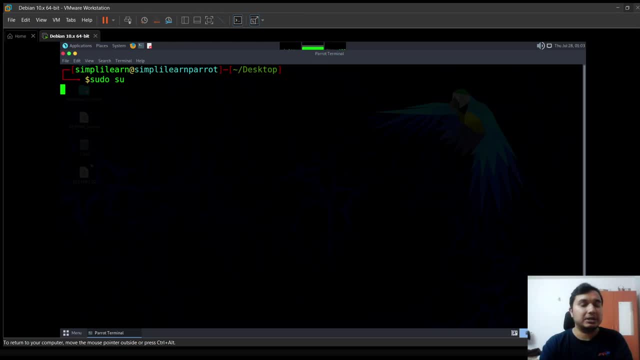 to use the sudo su command. This will turn our console into an administrator console. So let's say we want to use some drivers or some external adapters or anything that requires administrative permission. we don't have to use the admin password again and again. 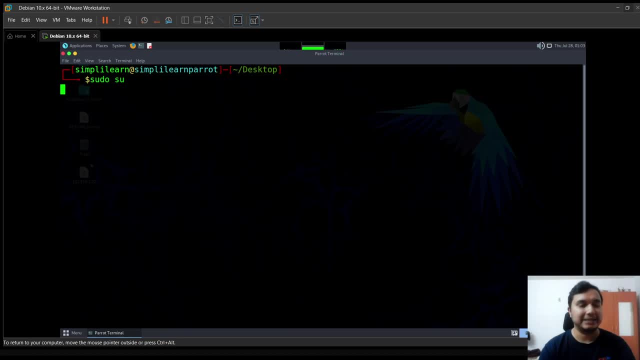 Just going to give it a bit of time, let me press the Merci button for it to recognize. OK, now that you see, this dollar sign has changed into a hash symbol, which means we now have root access of this console right now, of this terminal. 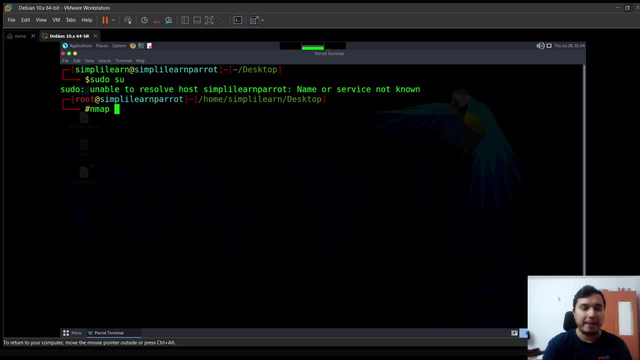 So what we're going to do for the ping sweep, where we have to check existing hosts, is we're going to use the command NMAP-SP And now they say 3P. We have to go to our console right now and we're going to run this. We're going to use the command NMAP-SP. We're going to use the command NMAP-SP. We're going to use the command NMAP-SP And let's go to the console right now. We're going to use the command NMAP-SP. 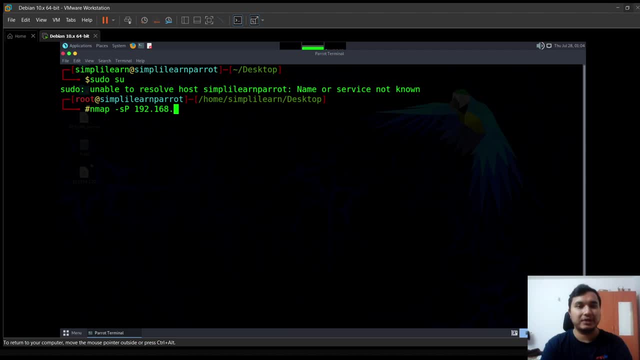 For the next command. we're going to use this command: go with the ip address of the current subnet that you're in, which is always going to be minus one, which all is going to be 192.168.1.1, the 24th. so this is going to take some time considering. 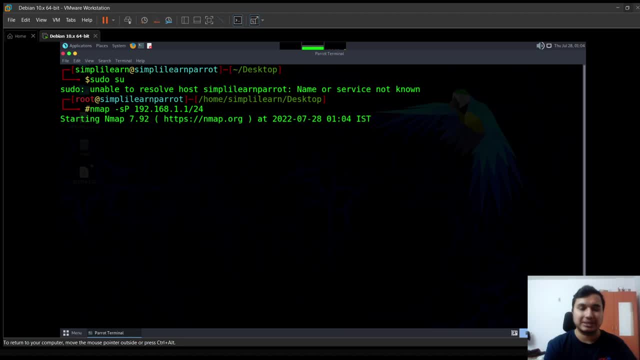 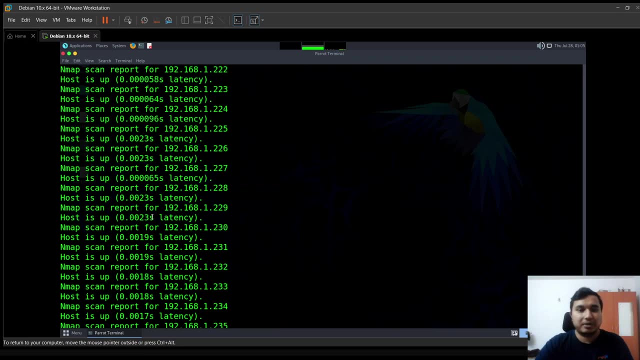 this is going to check all the hosts in this particular subject. the command then returns a list of posts on your network, which is this, and the total number of assigned ip addresses, if you can spot, like any ip addresses that you cannot account for in your network or your server. 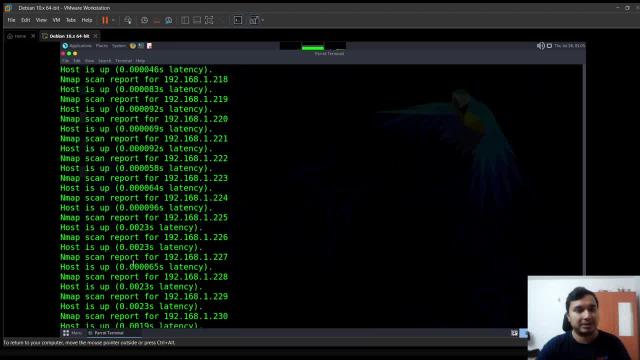 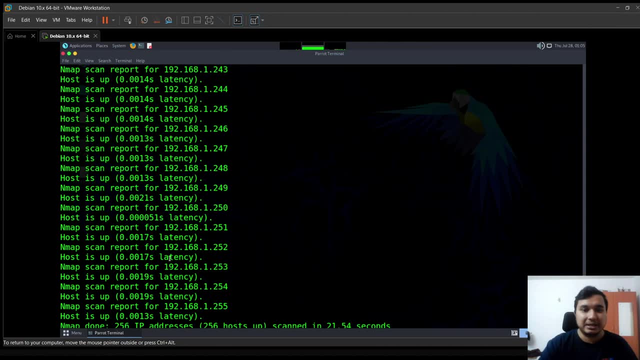 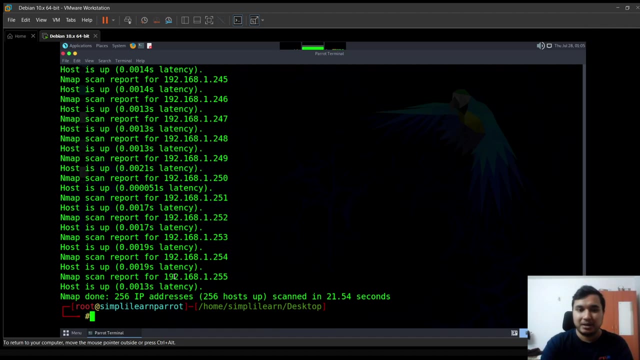 you can then further commands to investigate them further using nmap itself. now coming to another feature of nmap which is a very important usage is when scanning post and map commands can use server names, ip addresses or even ipv6 addresses. a basic nmap command will produce information. 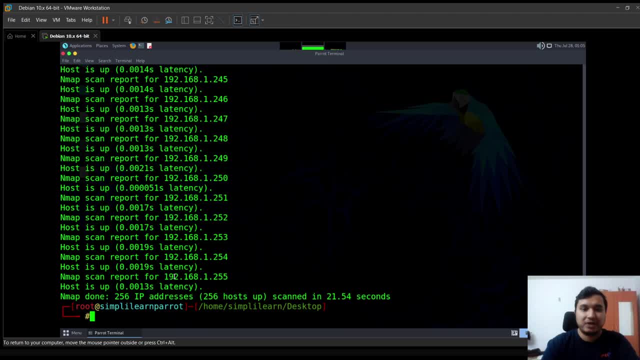 about the given host. so to run a basic port scan we can just use the nmap command. with the nmap command we can run a basic port scan. we can just use the nmap command with the ip address of the device or the ip address that we are targeting the port, now the host machine, that 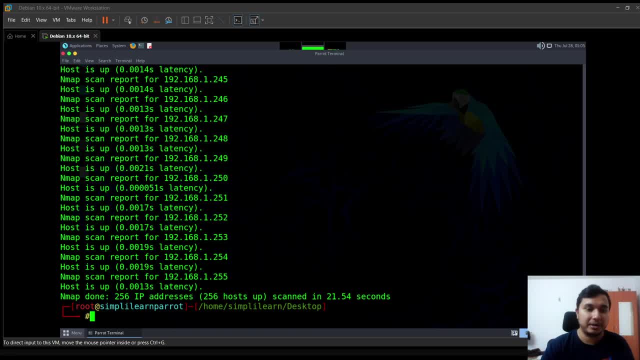 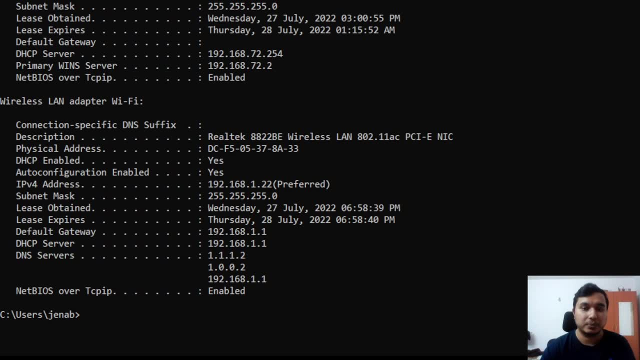 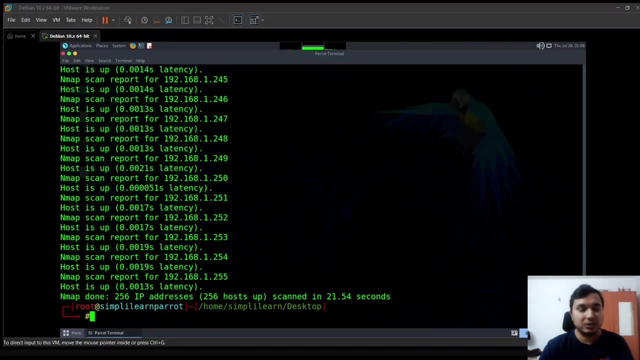 i am using currently as this current ip address. we can see the current ip address is 192.168.1.22 as it's written in the ipv4 address preferred section. so now we're going to try and attack this host machine using nmap on valid security operating system, so we're just going to go with the nmap. 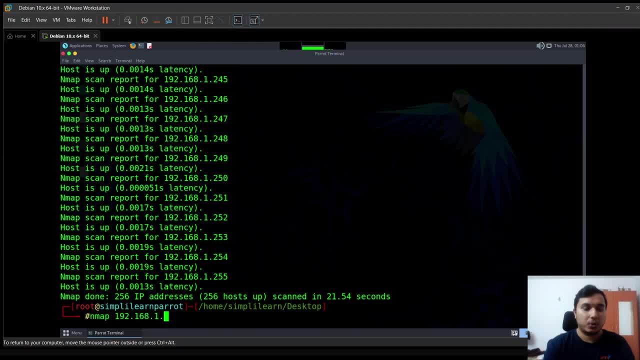 192.168.1.22 and press enter and it's going to start scanning the host for different services and the ip address that are that are being run on the system. the speed of these scans usually depend on how quick the processor is and also how quickly the two machines can connect with each other. but two machines, i mean the virtual. 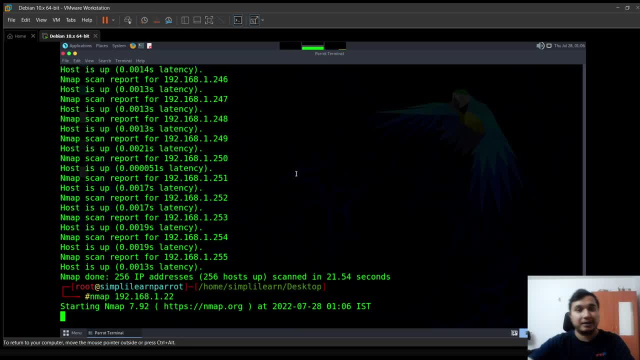 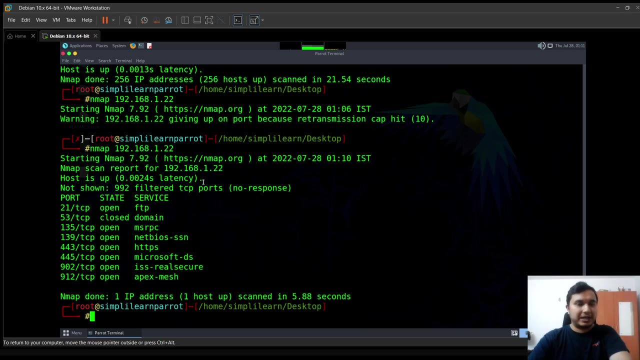 machine in this case and the machine that is being attacked, which is right now the post machine, that which is running vmware workstation. as you can see, the post scanning is complete for this particular ip address and you can see the number of ports is mentioned and the services that these posts are used for. 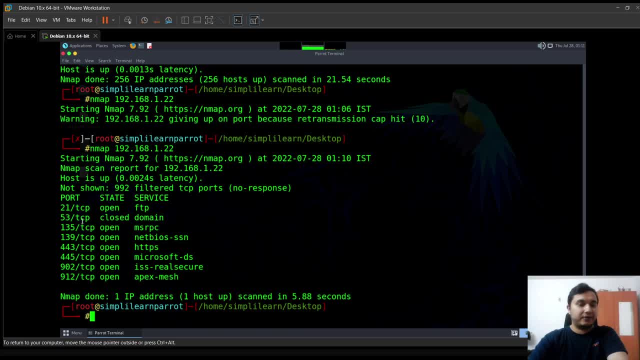 is also mentioned. it says which of these are open. for example, the 53 tcp port. we can see it is closed, while some of the other ports are open. now, one more feature of nmap is the ability to guess the operating system of the ip address that we are attacking. for that we need to. 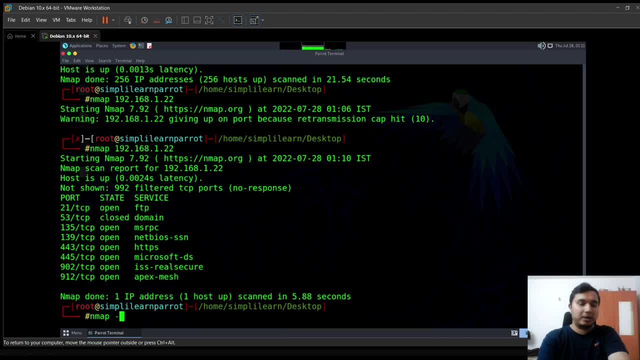 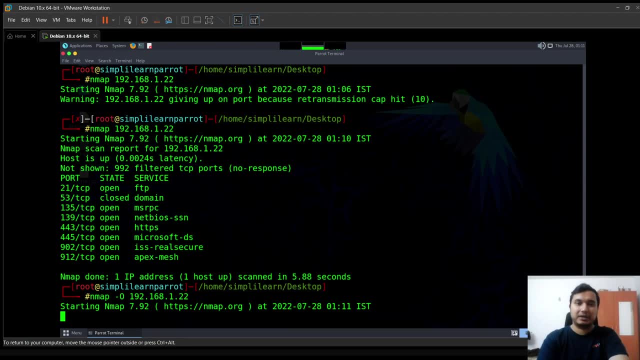 add one more flag which is going to go with. the normal command is nmap minus four and the regular ip address that we are in the process of attacking. let's give it a few minutes to run the scan and it will try and put a small guess on the operating system that this host. 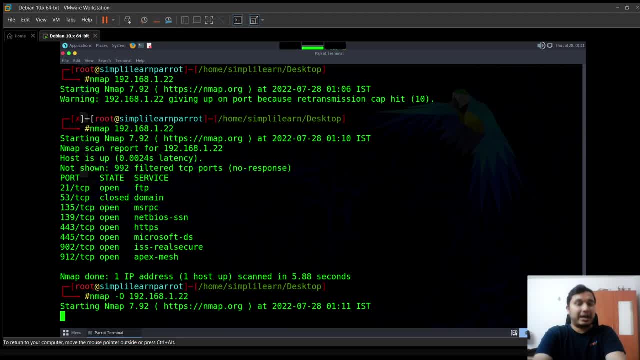 might be running. this guest might not always be accurate, but it puts a small idea and this is much more accurate in the case of actually unix based operating system other than windows based operating systems. it may be able to detect that if it is a windows or linux, macintosh and so on, but it may. have difficulty finding exact single versions, which will become easier in the case of linux, because we can identify different distributions by some of the kernels, which and most of the vulnerabilities comes from the kernels and not the particular distributions. as you can see, the os detection guess is complete and you can see aggressive os. 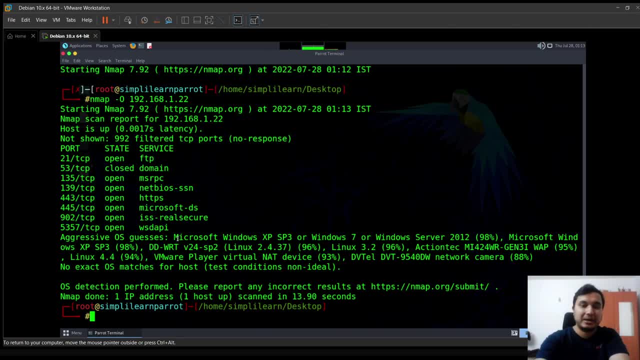 guesses over here, which is microsoft, windows xp service pack or windows server, and there's a 90 percent guess. that is mostly like i mentioned. if you can guess, if it is a windows based system, you can apply the vulnerabilities and the exploits accordingly. now, at times, you may need to detect. 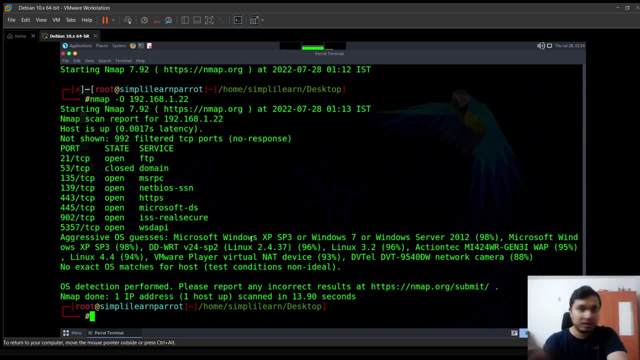 service version and the particular and similar information from these open ports. actually, this is useful for troubleshooting and scanning for vulnerabilities or locating services that need to be updated, considering a lot of the new updates are used to fix these kind of open vulnerabilities. so the flag that we're going to 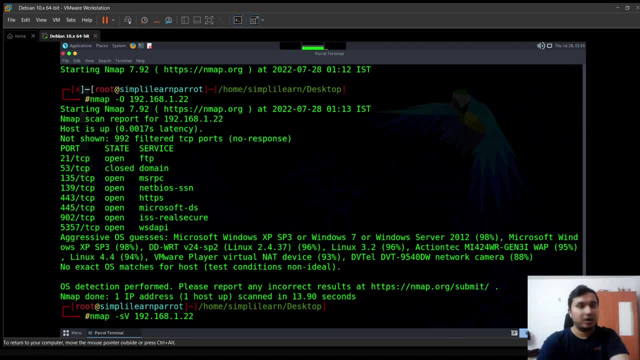 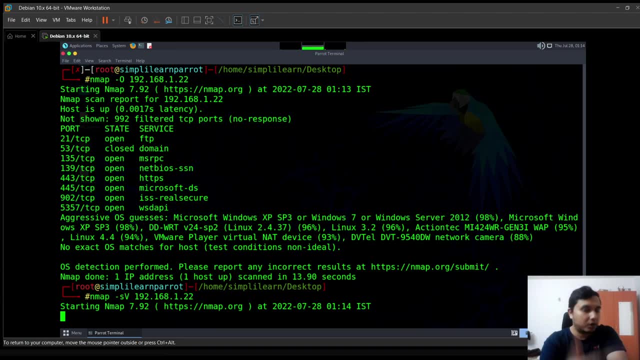 use in this case is minus s v or hyphen s v, because the only thing that's going to change with the nmap and the ip address of the host system staying consistent. a lot of the services that are being run on these ports are often not the most safe, for example. 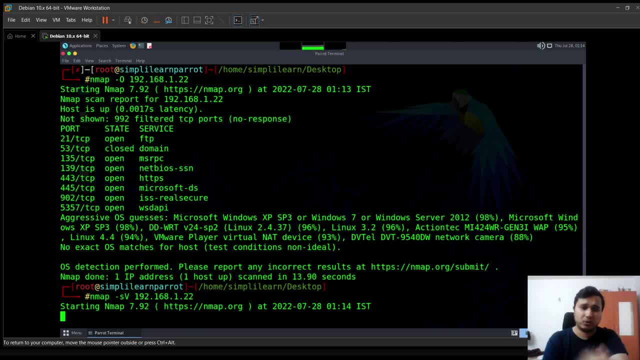 apache web server, which is a very common web server being used for even local and global projects. a lot of the older versions used to have systems that can allow privilege escalations or other vulnerabilities that can allow hackers to get into your system without even you getting a trace of it, so the updated versions tend to fix these as quickly as possible. 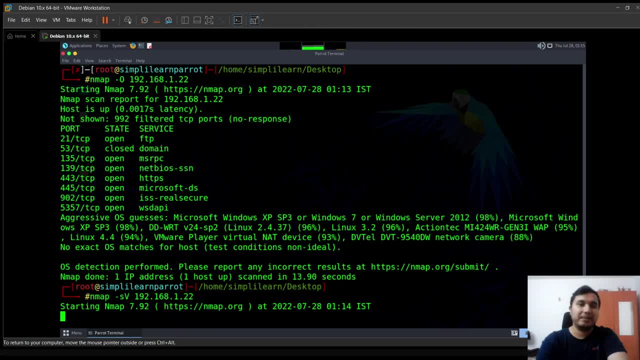 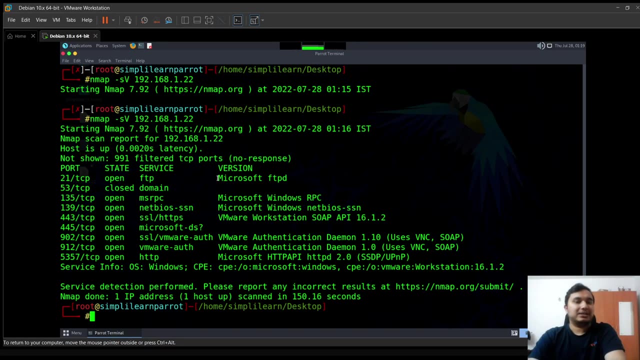 and most of these versions do not circulate in the real world but can be used for ethical hacking and testing on how these vulnerabilities, on how these vulnerabilities can be attacked further. now, with the sv command scan is complete. you can see that it is mentioning some of the versions of 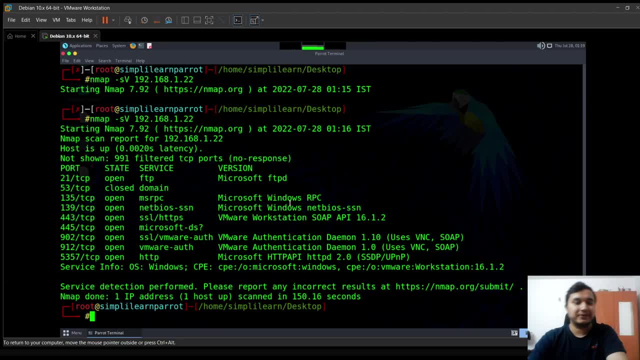 the services that are being run on the particular ports. once again, like i mentioned, using these version numbers you can identify particular vulnerabilities and use the exploits designed for these vulnerabilities to gain access to the system. another thing that nmap does well is port scanning. it's one of the basic utilities, actually, that nmap offers and, consequently, 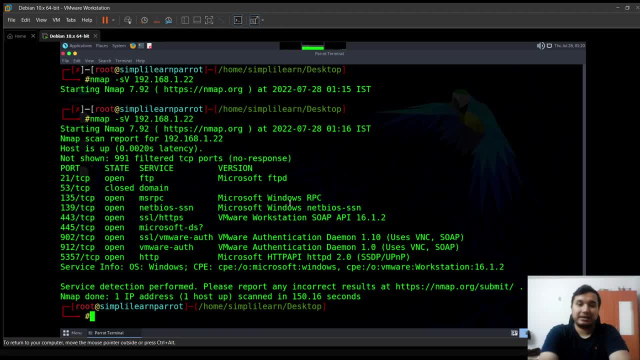 there are a few ways that this can be done, and one of the ways that it can be done is by using the port scanner, and using the port scanner, you can see that this command can be customized further. for example, to come to start a port scan, we're going to use the flag of my hyphen, p. we're 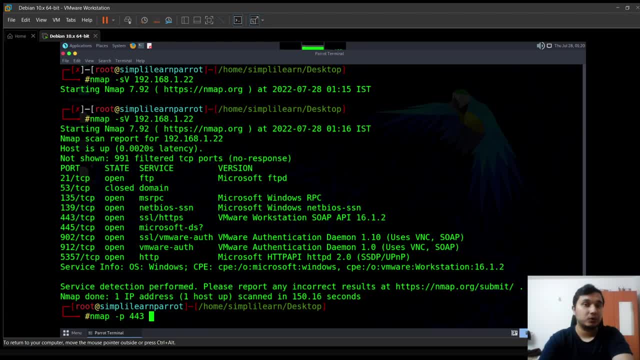 going to specify a random port, for example 443, which we know it will be open because it is the port used for https connections, which is obviously essential for you to access the internet, and, once again, we are going to use the ip address of our local host at the test machine that are being 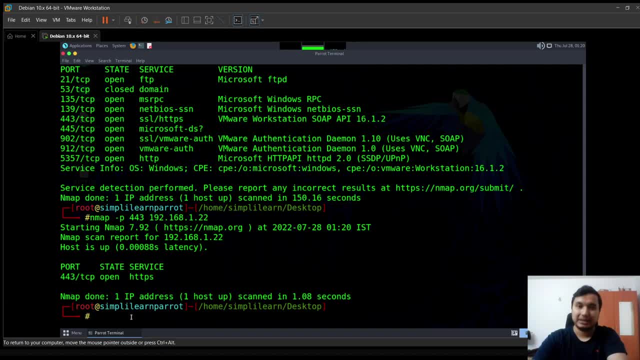 attacked, so we're going to use the ip address of our local host at the test machine that are being attacked. now you can use multiple ports. you can check multiple ports this way. for example, and map hyphen p, we're going to use scan- three different ports: 443, 80 and 445. 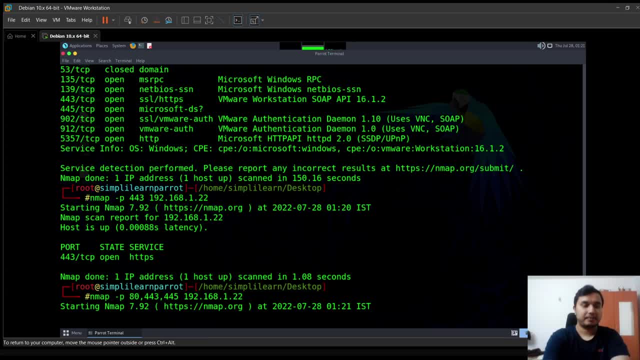 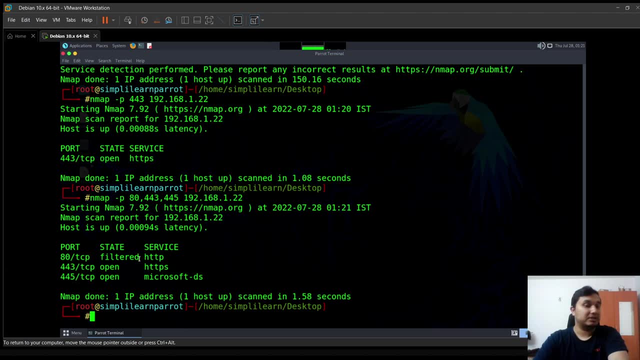 we use the same ip address again and it's going to show the state of all the three ports. now you can see this filtered part here, which which does not mean it is open and it cannot be exploited in any way, at least right now. maybe that there is any other service that is being run. it can be exploited further, but right. 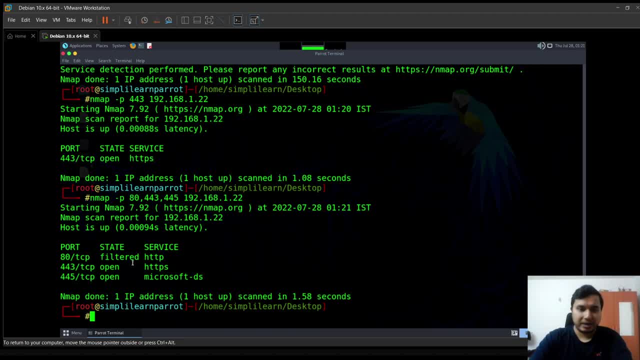 now it is in a filtered condition. that is how we can actually scan for multiple ports together. you can also. we can also use actually in a support scanning in a range format. for example, let's say we're going to scan the ports from 200 to 300. once again, we're going to use the hyphen p. 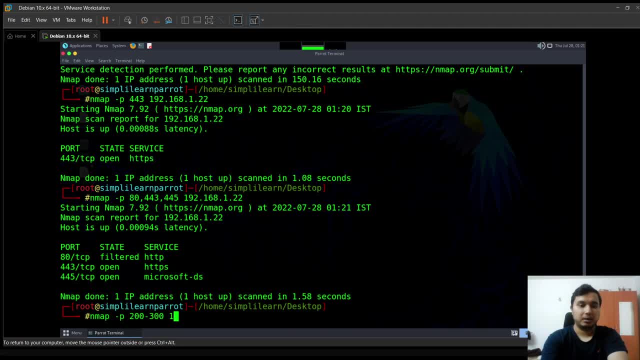 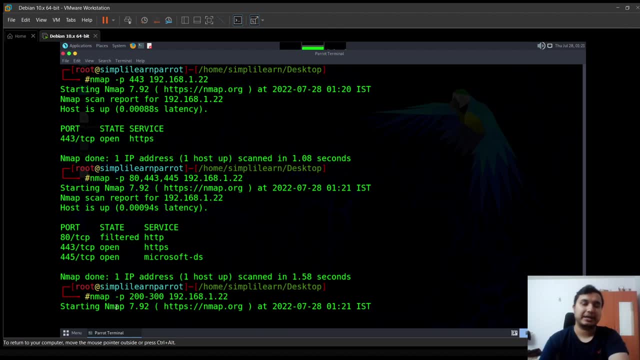 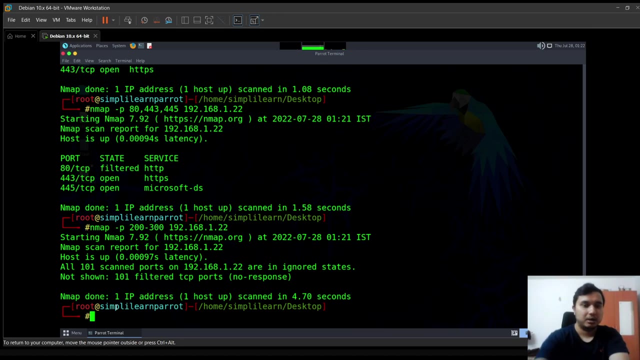 flag and then the ip address of the system being attacked. it's going to scan all the posts from 200 to 300 and mention what are the ports that are open, filtered or just straight up closed. as you can see, all the 101 scan ports are in ignore state. 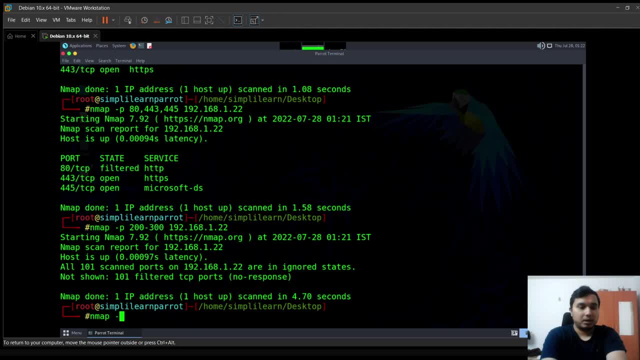 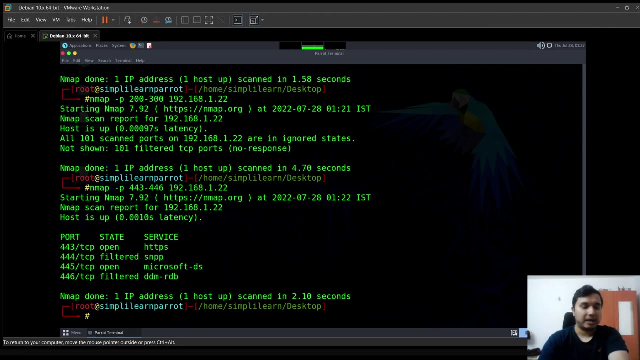 for example, if we try to scan a range in a more reasonable range, for example uh 443 to 446, that's it. we'll keep the ip address similar and you can see two of them are open and two of them are filtered for different reasons. this is how you can find out which of the ports are liable for exploitation before attacking. 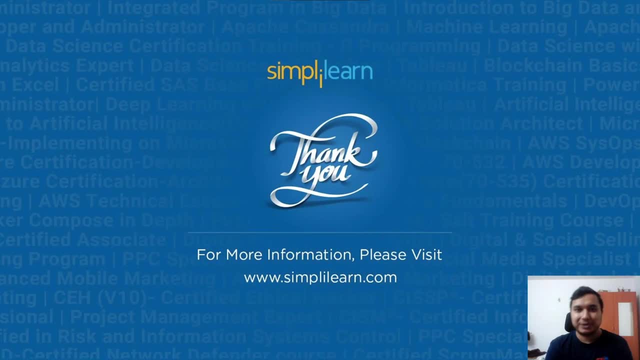 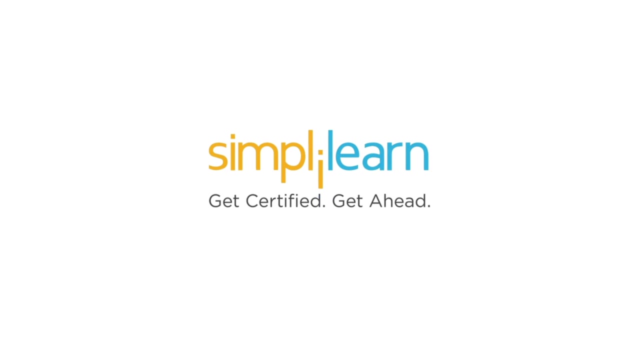 these kind of devices. hope you enjoyed this video. please let us know in the comment section if you have any issues with network security or the things that you learned in this video. subscribe to our channel for more videos like this and thank you for watching hi there. if you like this video, subscribe to the simply learn youtube channel. 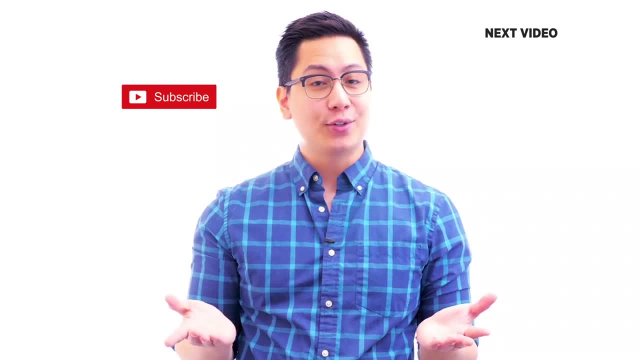 and click here to watch similar videos. to nerd up and get certified: click here.